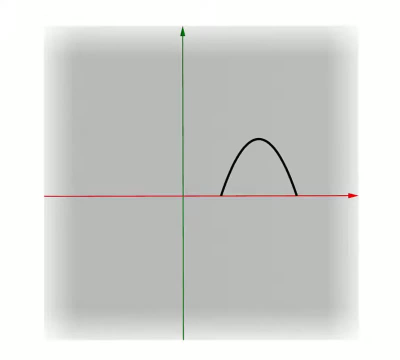 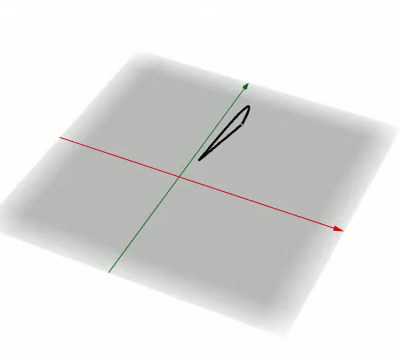 I want you to imagine that you have a portion of some graph on a piece of paper in front of you and that this graph is cut off at the x-axis. If we spin this graph around the y-axis, it will outline a shape. Can you see what that shape is? 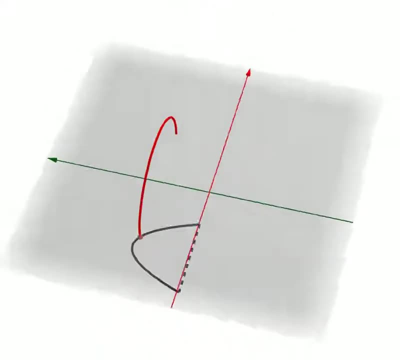 To get a better idea of what's going on, let's follow a single point on its journey around the y-axis. It just makes a circle. In fact, any point that we choose to follow will just make a circle, since the graph is actually spinning in a circle around the y-axis. 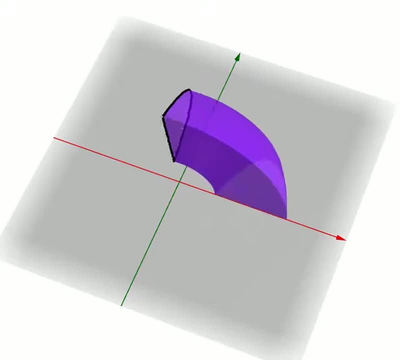 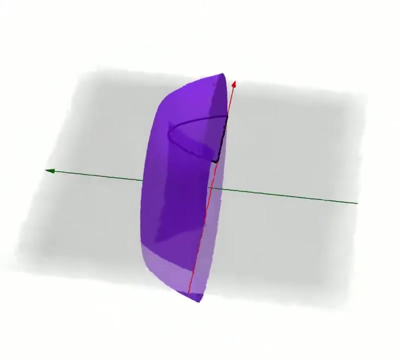 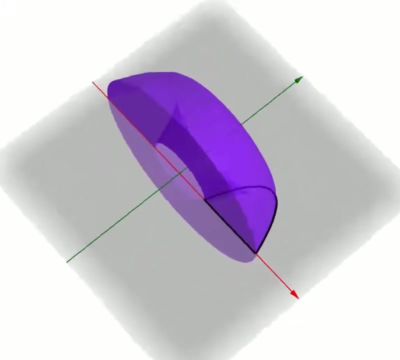 Now take a look at the path of the entire graph. as it spins, It looks like a dog bowl with a hole in the bottom. My question is: what is the volume of this three-dimensional shape? Before we answer that, let's follow a thin rectangle. 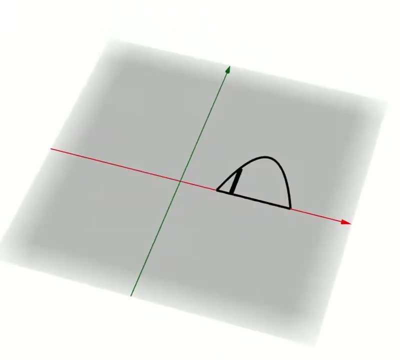 as it spins around the y-axis. If you're thinking that this looks like the setup for Riemann sums, you are absolutely correct. Unlike the other three-dimensional shapes, Riemann sums are a set of three-dimensional shapes. Unlike the previous video on disks, this rectangle actually traces out a cylinder which is just 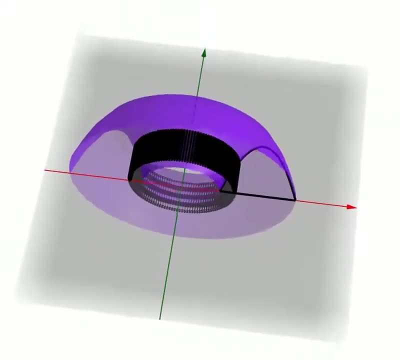 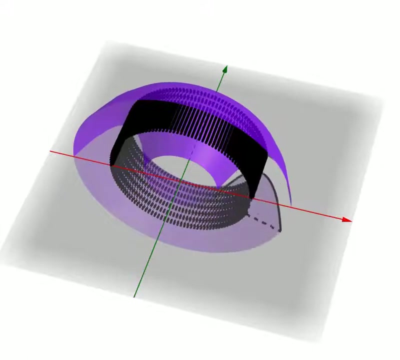 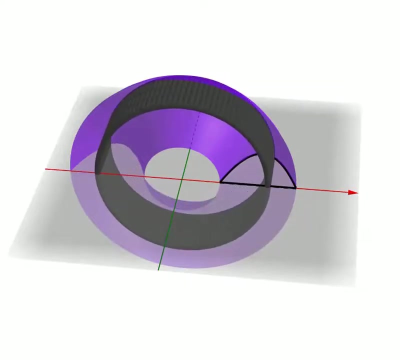 a fancy term for the side of a soda can, And if we follow a different rectangle we just get a different cylinder. Here's a look at all the different thin cylinders we could get by following the path of a spinning rectangle. This may give you some insight into how we will formulate a systematic way. 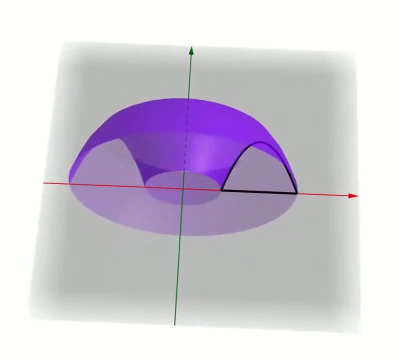 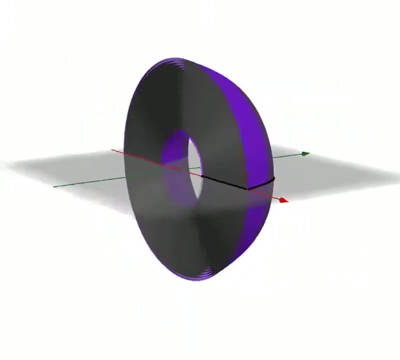 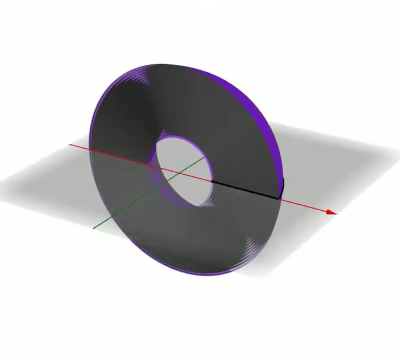 to calculate the volume of this entire solid shape. If we had a bunch of different sized cylinders which were all insanely thin, we could cram them into this shape and add up all their volumes to approximate the volume of the entire solid. And, of course, the thinner our choices for cylinders, the better our volume approximation. 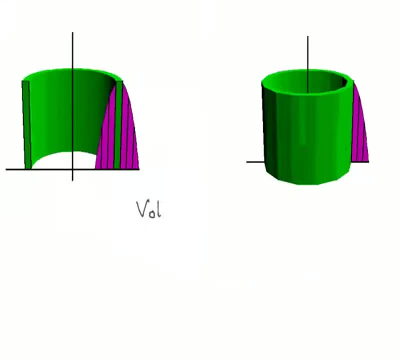 would be Time to tackle the math happening behind the idea. We will first find the volume of a single cylinder. These are also called cylindrical shells, or just shells for short. The volume of a super-thin shell is going to be the base times the height times the. 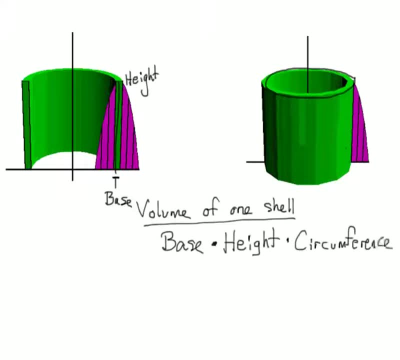 circumference of that cylinder. I'm actually lying a little bit here. I want to see if you can figure out what my lie is. And actually, the thinner these shells get, the less I'm lying. So that's good, because these shells do get crazy thin, so it's totally okay.